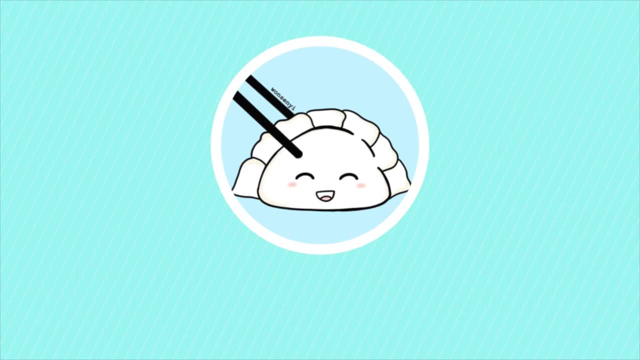 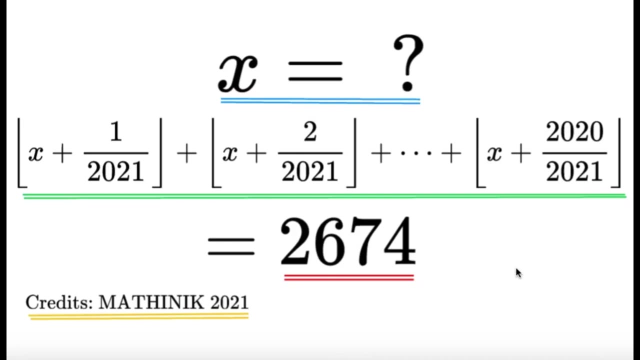 Hello, hello, it's Template here. Here's an item on algebra. Find all possible values of x such that the green expression over here is equal to 2674.. Now credits to the Matinic 2021 for this item. As usual, pause this video if you'd like to give this item a try, But 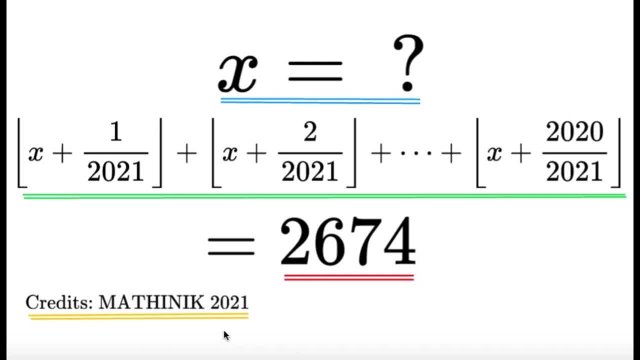 if you're done, let us dive into the solution. Now here we have 2020 floor functions and it's not really easy to kind of solve for x or try to remove the floor functions one by one. So what we're going to do here first is to make an observation. 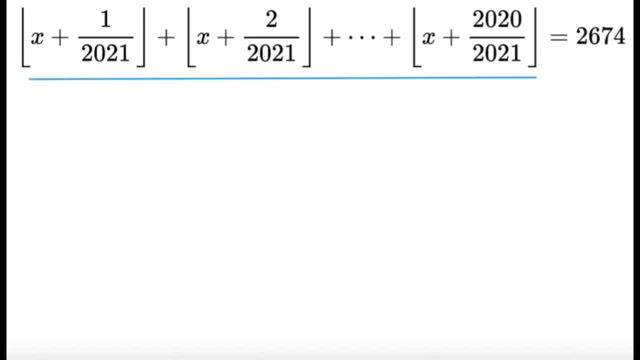 Well, obviously, there's a pattern: x plus 1 over 2021,, x plus 2 over 2021, and so on. But what's important here is to realize that well, let's try to see the smallest value. 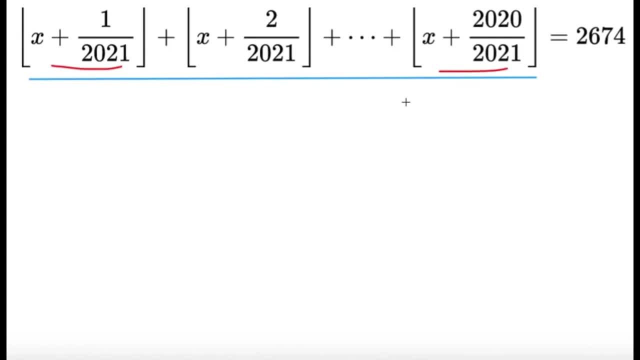 here and the largest value here, that is inside the floor functions. Take note that if we take the difference of those two numbers- so if I take the difference of these two numbers, it's going to be 2019 divided by 2021.. And what's important about this is that it's less. 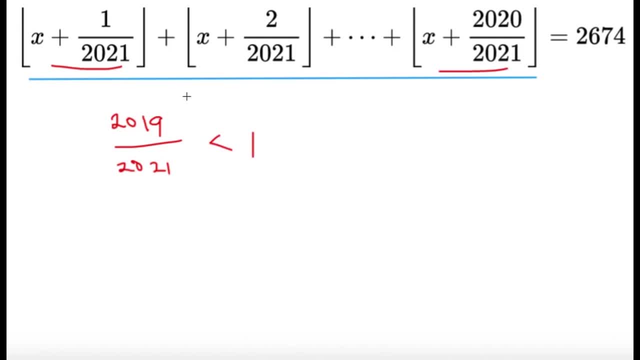 than 1.. And there is a nice result following from the fact that, OK, the smallest and the biggest numbers have a difference of less than 1.. Now, what this is going to tell us is that, well, there are 2020 floor functions here, but there can only be, at most, two different. 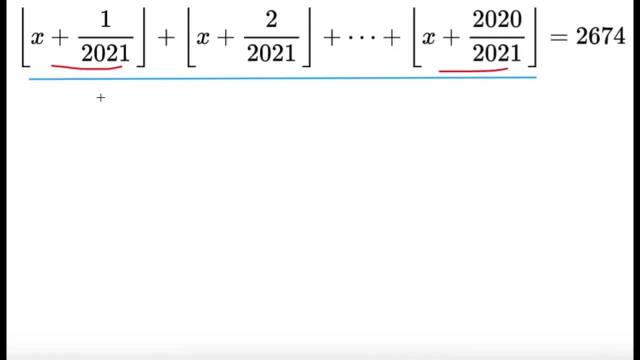 values for among all of these? because, well, these two, the thing inside, they differ by something that's less than 1.. So it's impossible for us to get the difference. So for this one, let's just say, let's say this is k, This can only be also k, just in. 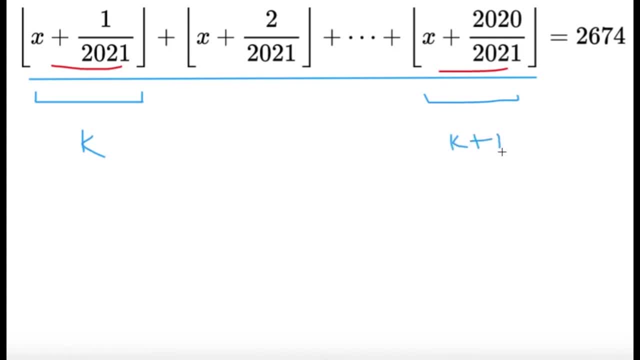 case It might be possible, It can be k plus 1, just so that, or like it so happened that, for example, let's say, the red terms are actually. let's just say, if the red term here was, let's. 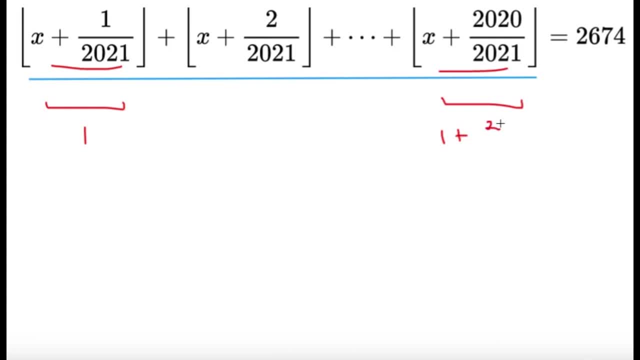 just say 1, then the red term here would just be 1 plus 2019 divided by 2021. And they'll have the same floor functions or like, yeah, they'll have the same floors. If it was something like 1.5, and then this would be 1.5 plus 2019 over 2021, that's certainly 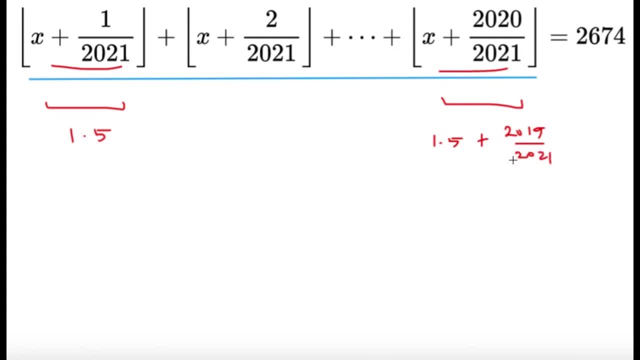 greater than a half. So the floor of this one would be 2, something like that. But it's impossible for any two floor functions here to have- sorry, any three of these- to have two different values because of the fact that, well, the smallest and the largest, they only. 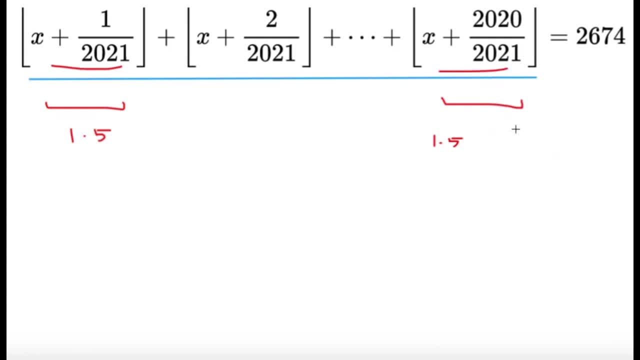 have a difference of 2019 over 2021. So we now have just two cases here. It's either all of them are the same, either all of them are the same, or some of them will be one value and some will be. 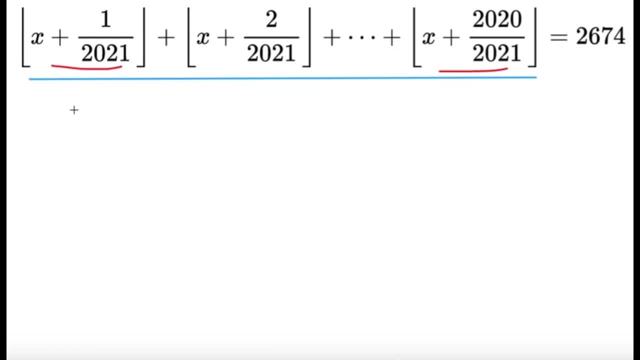 the other. So let's talk about the first case. Let's just say case one. all the floor functions are the same. So if that's the case, well, it's just a matter of kind of letting what each of these will equal to. Let's just say one equals. each of these equal to k. Add 20,, 20 of these. 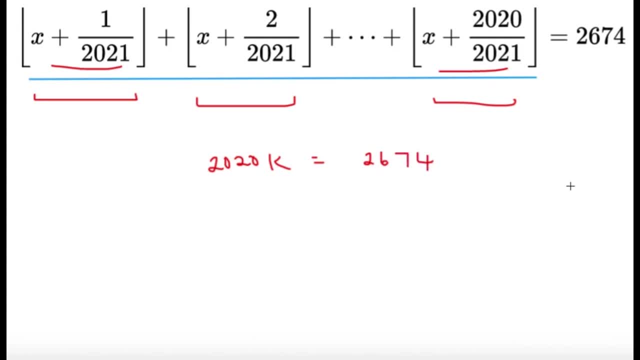 Well, the restriction here is that k is an integer. So well, 20, 20 times k, that's going to equal to 2,630.. I can, I mean I can, solve for k, but obviously k will not be an integer in this. 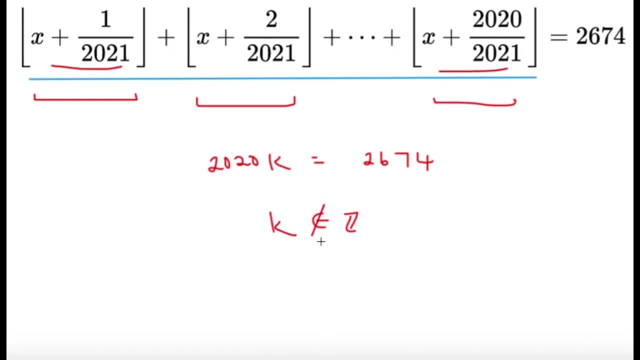 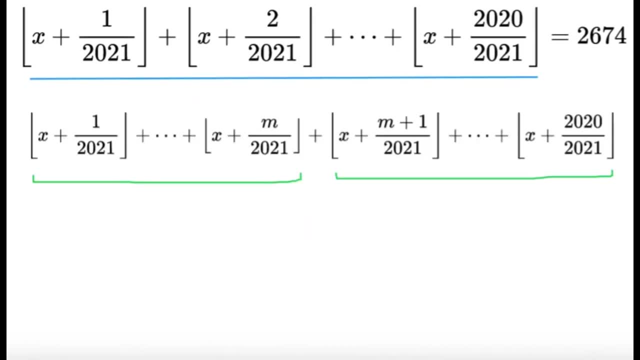 case. So in this case I think it would be impossible here for us to have, like, all of these floor functions to be of the same value. So let's move on to the next case. Let's just say some of them has a floor function of a certain value. Let's just say k for now And the other. 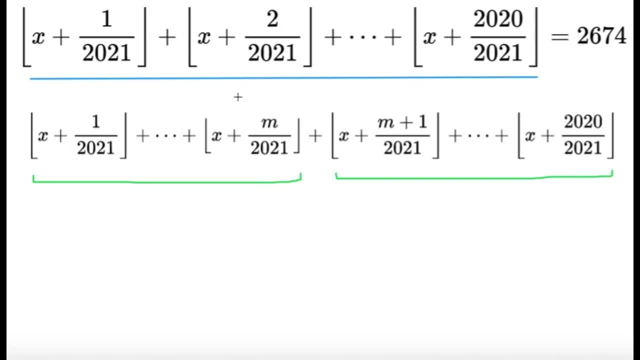 set would have a floor functions of k plus one. So let's just say that the floor of x plus m over 2021 and the floor of x plus m plus one divided by 2021, let's just say they're different, So like: 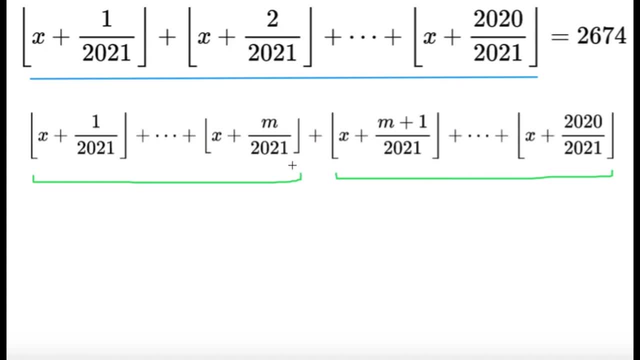 this value. let's just say the floor of this value is k And obviously that's going to be applied to all the terms here, because they should be. they should have the same floor functions of k, because m here, based on how we. 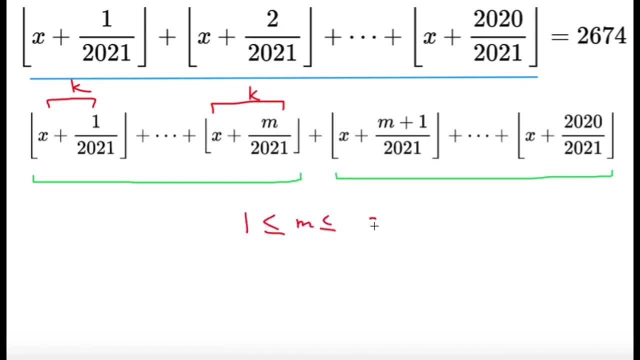 define it. it's going to be between m, should be between one and 2020.. And well, here the values here should be k plus one, the next possible integer. So here we just have a floor function, some of which are equal to k, some of which are equal to k plus one, and they're separated here. 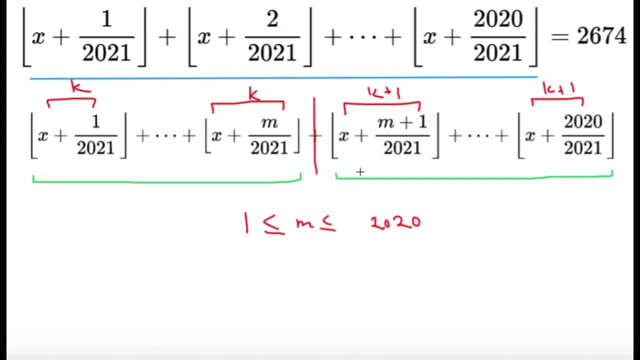 actually between these two terms. So now it's just a matter of writing this in terms of k and m actually. So let's talk about the left part. So I have how many terms here? I have m terms, because I started from one over 2021, and I did it until m over 2021. So that's gonna be total. 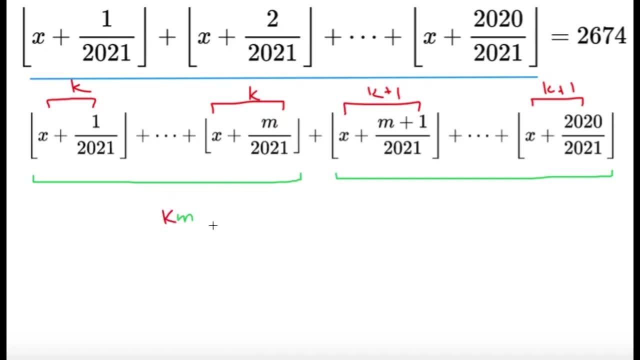 of m terms. Each of them has a floor function of k, so that's km, Then I'll plus. now we can just do complementary counting. there are 2020 terms in total and there are m terms, So if I add one by one, there are 60 terms, which has a half of the s squared. With that being said, we usually just add each term and add an extra one to the s squared, and that adds the board over the other part, and it mucho 아니라. 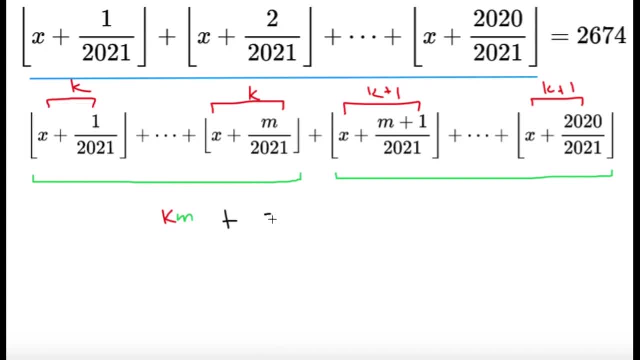 in this part. so there's going to be a total of 2020 minus m terms here. All of them has a floor function of k plus 1.. And well, this is the sum, and this is apparently equal to 2674.. So this sum over here, we just kind of evaluate this. 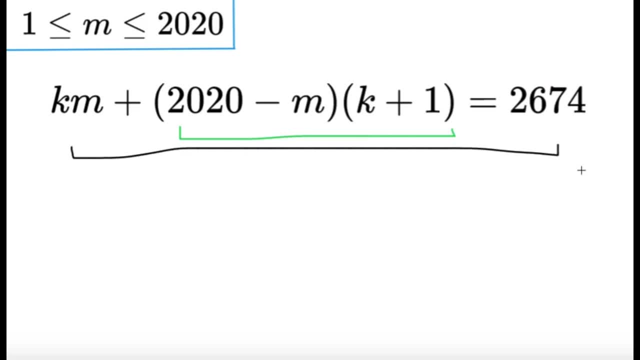 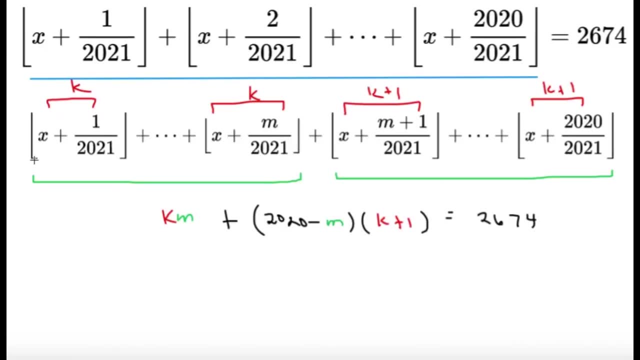 one, and this will now be a Diophantine equation in terms of k and m. So we know that k and m must be integers, because k is the floor function of, k is the result of: well, k is an integer, so it's the floor function of these values, and k plus 1. 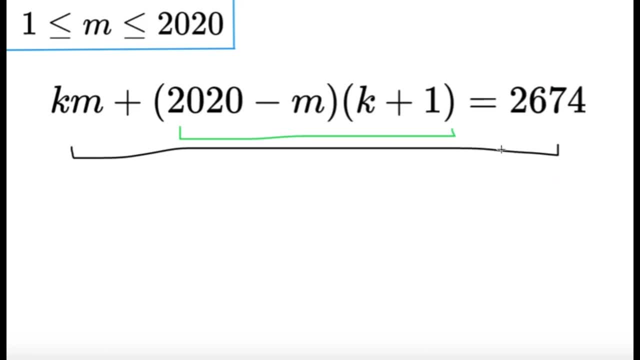 is the floor of these values, So we just have to solve for integer values of k and m. So let's try to expand this one So just 2020k plus 2020, minus mk, minus m, And then, well, mk is just km anyway. so there we go, So km and then minus km here. 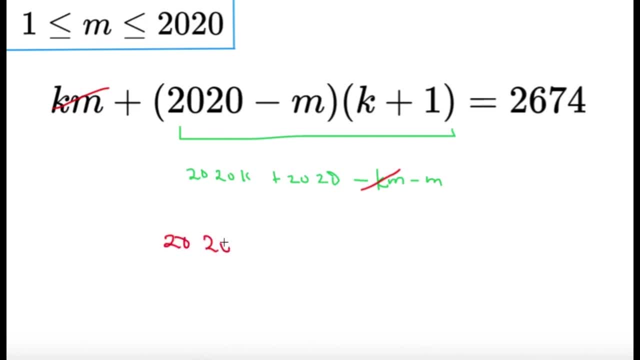 cancels out. so I'll have like 2020k minus m. that's going to be equal to well, this 2020, I can subtract it from 2674 and I'll get 654 from there. So I have 2020k minus m is equal to 654.. Now we 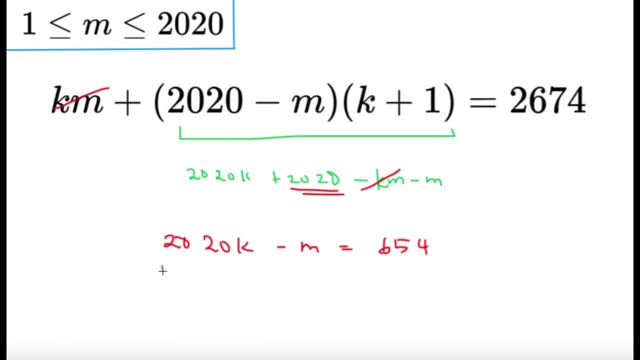 know that m lies between 1 and 2020.. So it must be the case that k equals 1, because, for example, if k was 0, m would be negative. Now, if k equals 1, m is possible, But if k equals 2.. 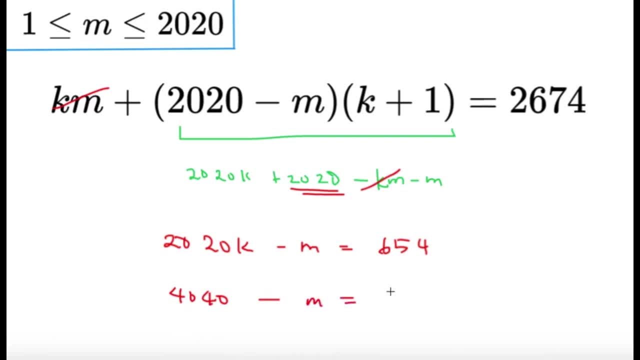 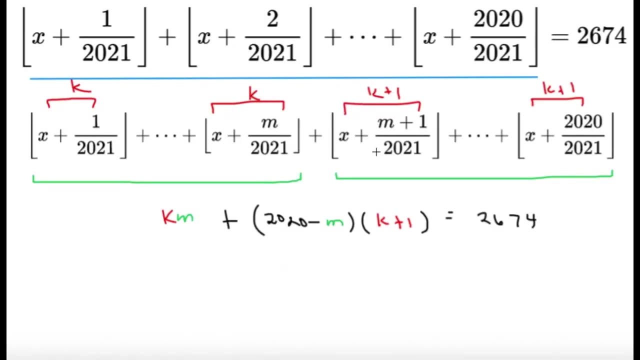 actually it's going to be 4040 minus m, being equal to 654, but m would be less, n would be 3000 something. so that's impossible. so with this we know that k here must be equal to one, so that m would satisfy this, which is the restriction for uh, the way we kind of set up uh m. so we know that. 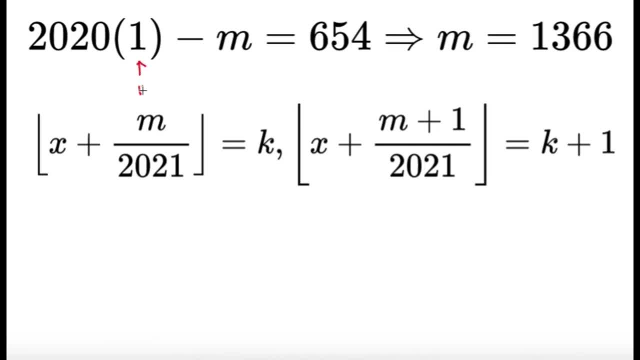 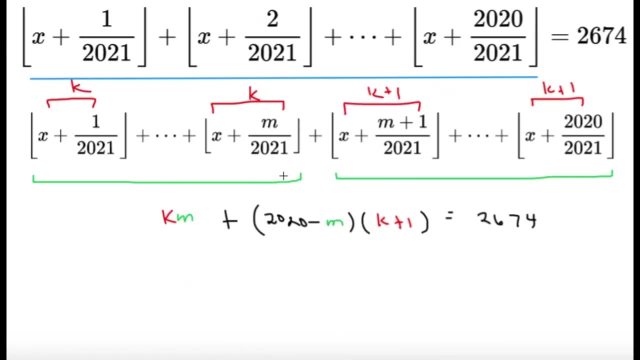 k must equal to one. we substitute it here, so k equals one and we have to solve for m. so solving for m it's just a matter of uh, simple algebra we're gonna get: m is 1366. so with this, since we kind of made the assumption that it's uh, these two are correct based from this. so we just kind. 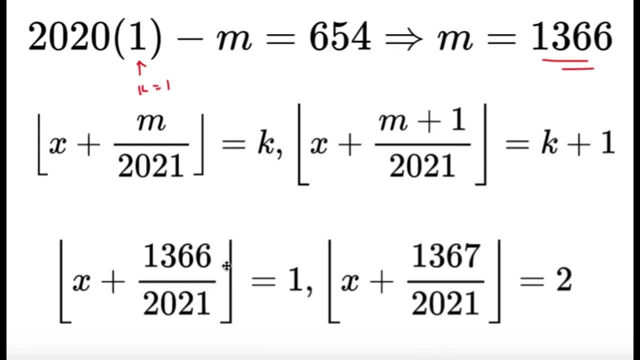 of substitute them. we know that x plus 1366 divided by 2021, that's going to equal to 1, and x plus 1367 divided by 2021, that's going to equal to 1 plus 1, that's 2.. now it's just a matter of. 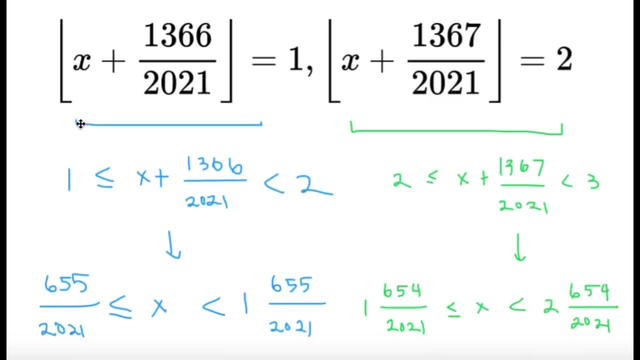 solving for x. now, these two floor functions will give us these two. so we know that the expression inside, if that's equal to one, that must be greater or equal to one but less than two. and similarly for this one x plus one, three, six, seven over two, zero, two, one that must be between two and three. 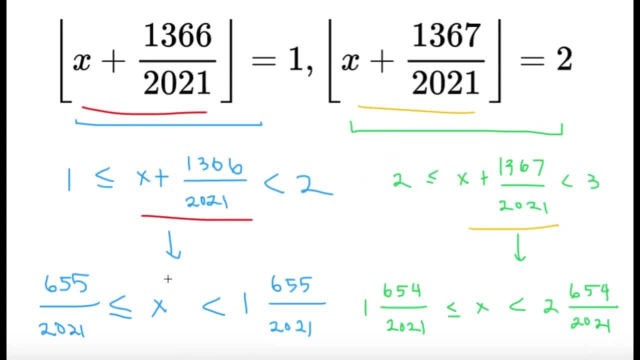 so it must be greater or equal to two, but less than three. we have to solve for x here. now. these will be the two inequalities for x, and the last step is just simply simplifying it and just kind of working out the intersection of these two, because we want these two to be correct. uh, yeah, we want these two to be. 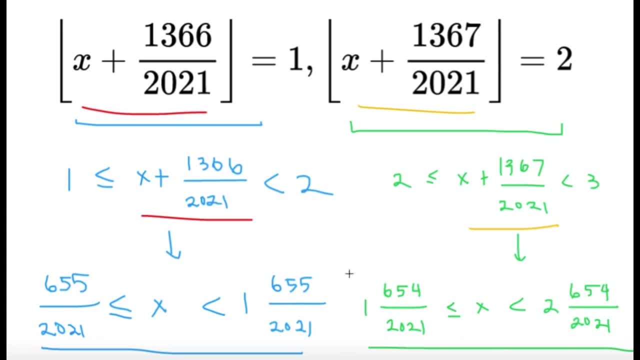 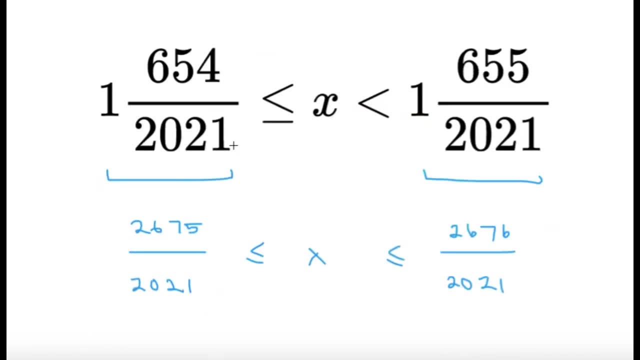 correct. so there will be a restriction and we kind of realize that the intersection it's going to be well: values of x greater than or equal to one and six, five, four over 2021 and values of x less than one and six, five, five over 2021. and there we have it now. if you want the answer in